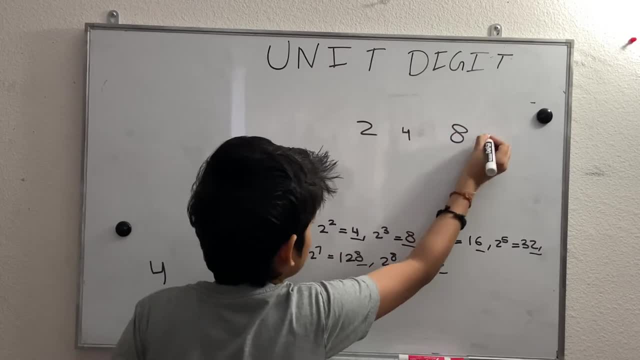 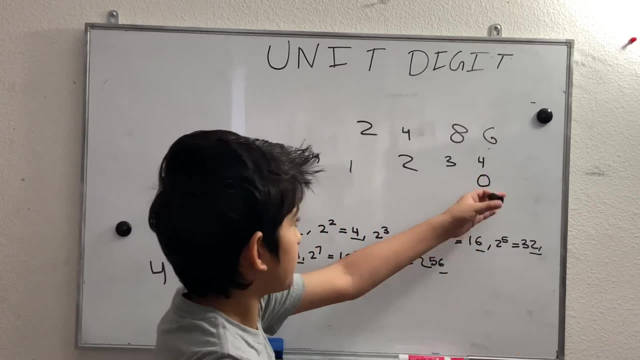 this is two. Let's give the value: of this is one, this is two, this is three, this is four, But four is also equal to zero, because it's going to be zero one, two, three, four. zero one, two, three, four. 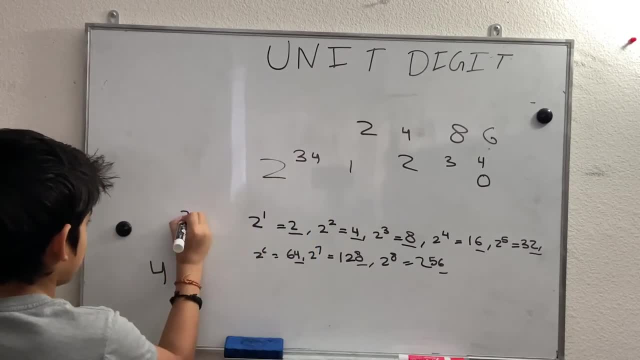 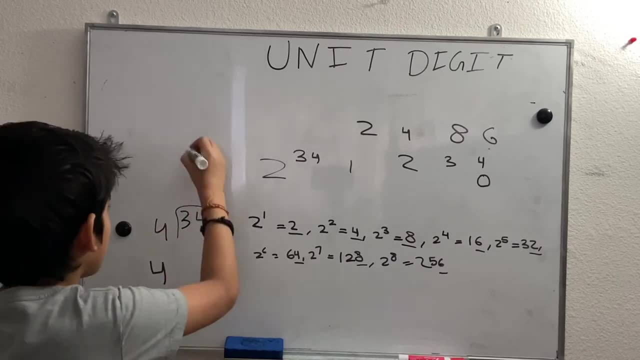 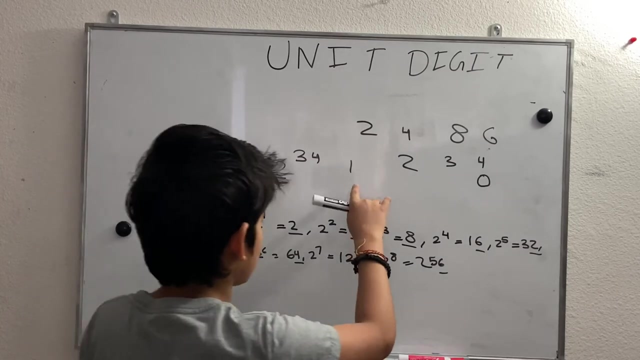 Okay, so now let's divide 34.. It's just, we don't need to do that. We get eight and we have to work with the remainder, And the remainder is equal to two. So now let's check which value is two, One? nope, it's just one. 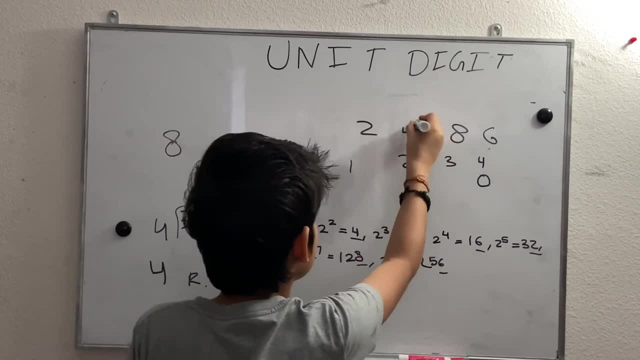 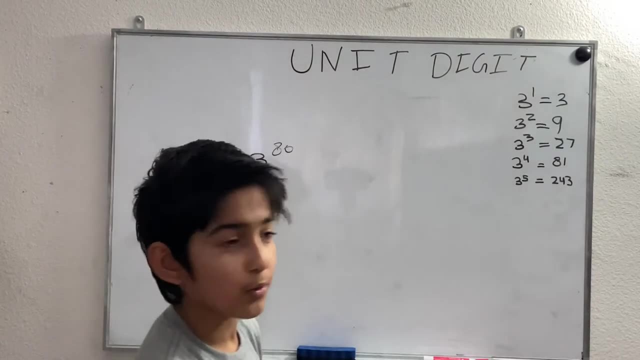 two. yes, So that means our unit's digit for this is equal to four. Let's head into another example of three to the power of eighty. So I wrote down: three is power one, so three's power five right over here. So one is three, three's power. two is nine, three's power. 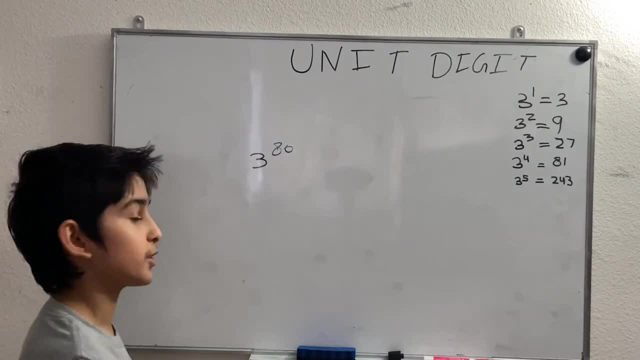 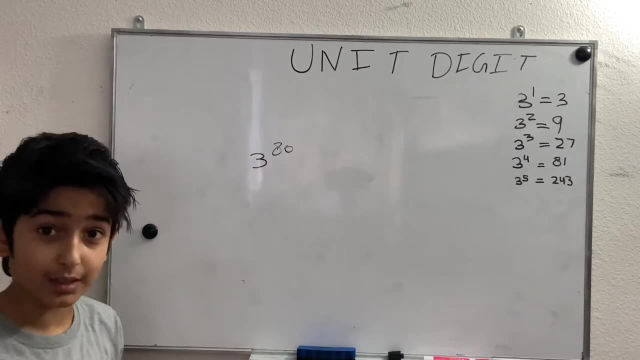 3 times 7 is 3,, 4 is 81, and 3 times 5 is 243.. I don't want to go any further because that's all I know, and otherwise I have to fetch a calculator. So why can't you just do this with a calculator? 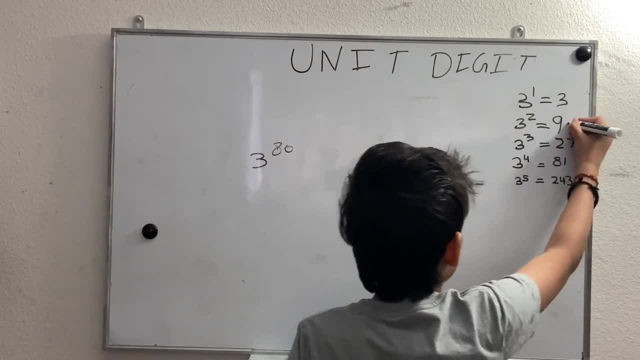 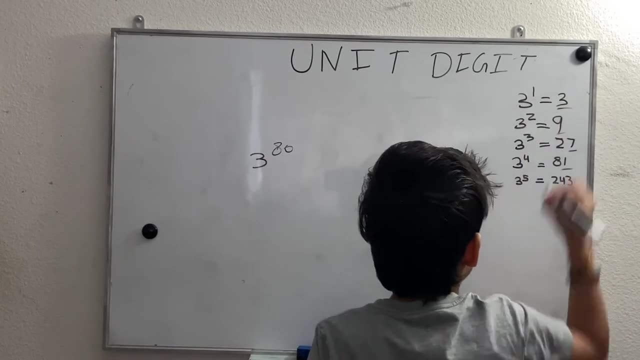 Okay, so now let's find a pattern: 3,, 9,, 7,, 1,, 3.. Because these are all the units to do right here. Now, if you multiply 3 by 3, because I don't want to multiply- the whole number is 9.. 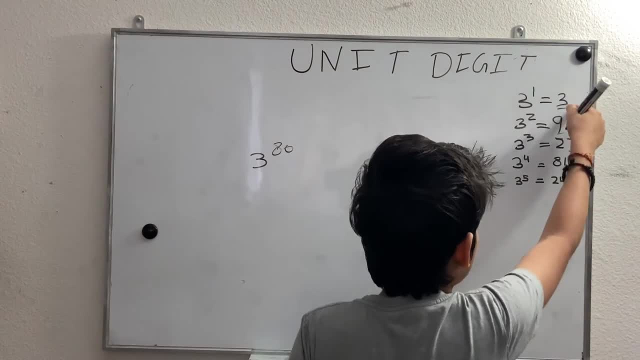 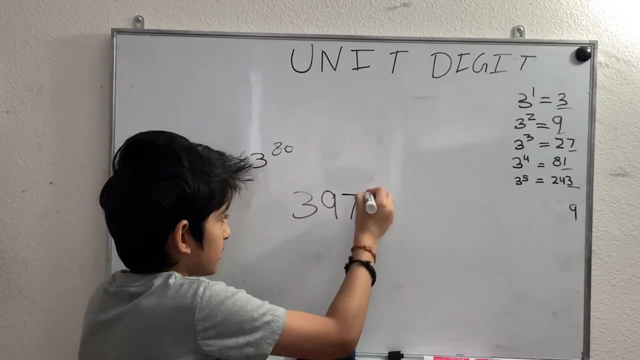 So now you can see the pattern is repeating: 3, 9, 7, 1,, 3, 9, so on. Okay, so we have the pattern of 4.. Let's just write it: 3, 9,, 7,, 1.. 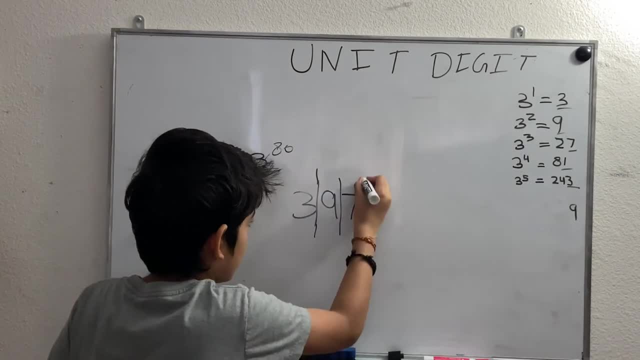 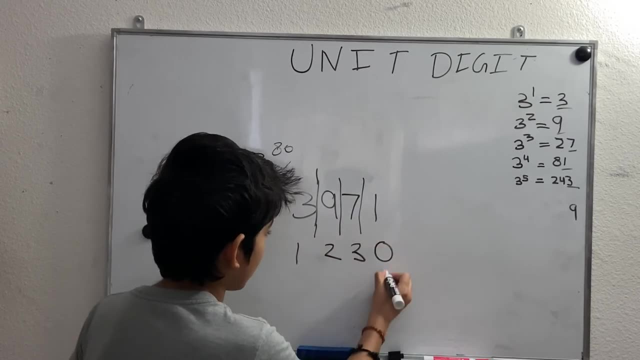 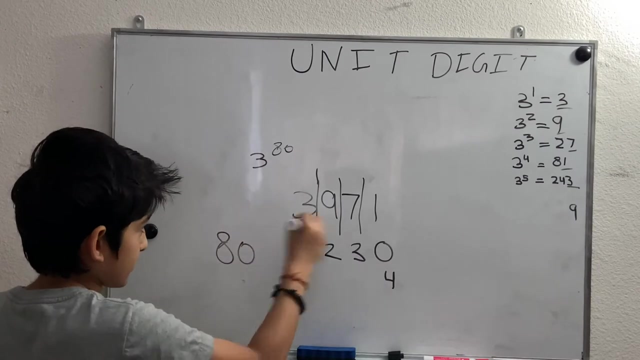 So this doesn't look like a 4-digit number. I'll just do separators. This has 1, value 3,, 0, and 4. Keeps repeating. So now let's divide 80 by 4, because there's 4 numbers. 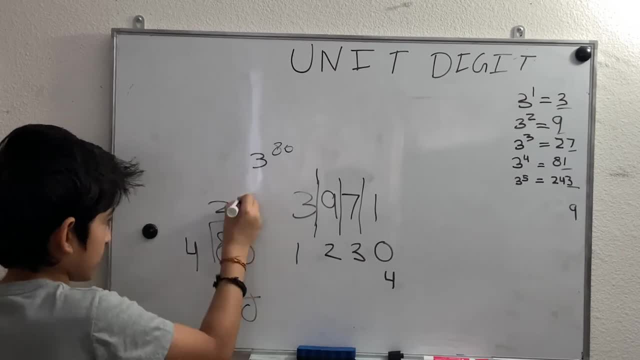 There's a 4., 1., 2., 3., 4.. You have a 4., 2., 3., 4., 5.. Did you get any numbers in there? No, I did not. Who can tell you? 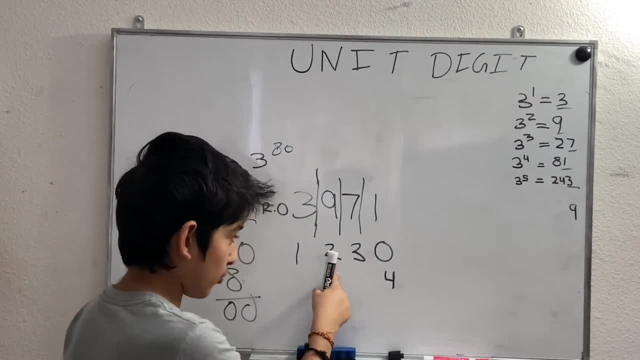 Okay, so the answer here is 4.. So the answer here is 1,, and that's the number that needs to be multiplied: 4., 5., 6., 7., 8., 9., 15., 20.. 21., 22., 23., 24., 25., 28., 29., 30., 59., 30., 32., 31., 31., 32., 33., 34., 35..